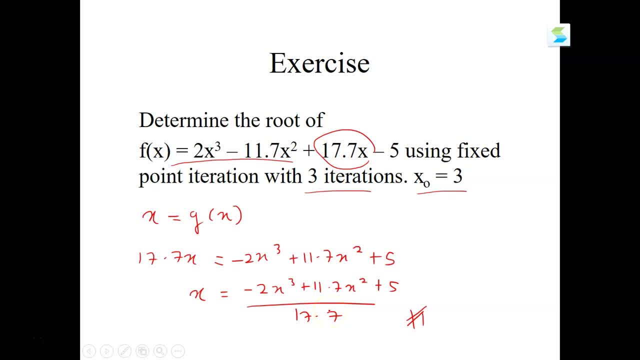 Either you know the error will converge or the error will diverge, Because you know you can have many other forms of gx. using this x, using this x. Okay, three types of equation In order for you to decide whether this is the correct equation. 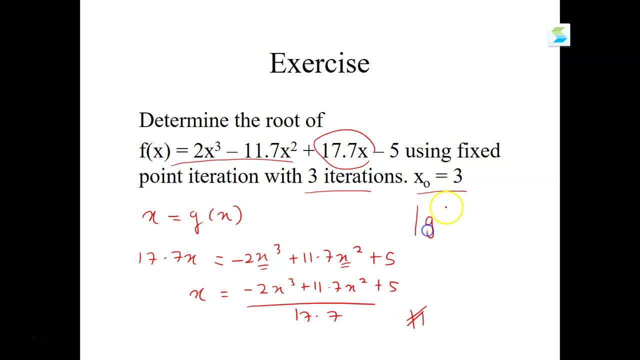 Or not. So you just work out the first derivative of the gx And make sure that the value of this first derivative, when you substitute 3 into the first derivative, Whether it will give you less than not 0, sorry, 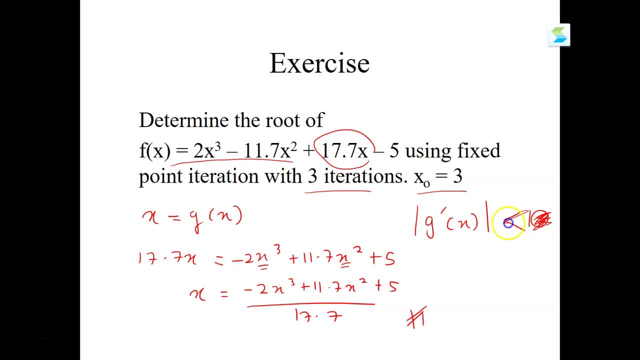 Less than 1 or not. Okay, not 0. It's less than 1.. It must be less than 1.. If it's more than 1, the error will diverge. So I have calculated this And, if you try on your own, find the first derivative of this equation. 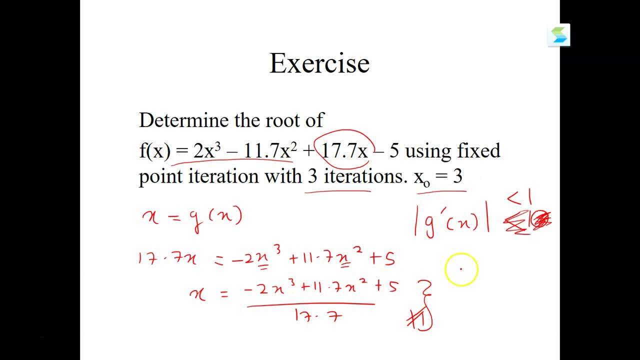 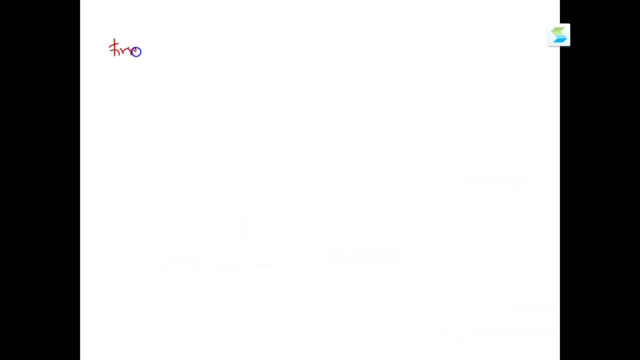 And then substitute 3 into the x's, Alright, You will get your answer: less than 1.. So this is good to go And we can proceed. So first iteration Alright, In which I will call it: x1 equals to. 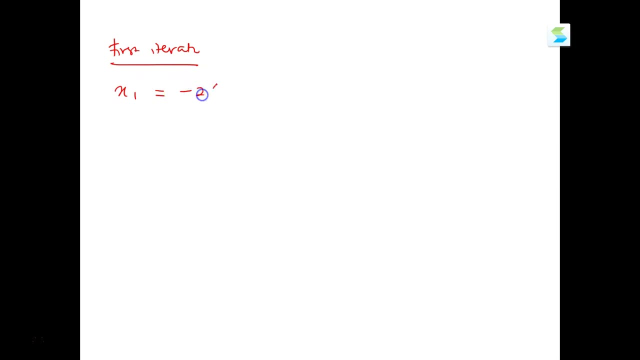 This is the gx. This is the gx Formula just now: Negative: 2., 3.. Okay, why 3?? Because we're starting. We're using the starting value of x, Which is 3.. So 3.. 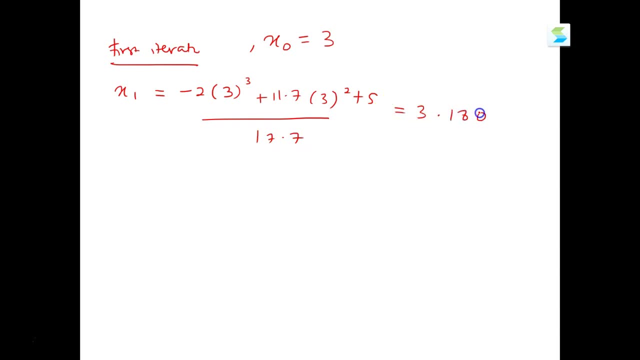 And you will get 3.180791.. Okay, of course the question Does not require you to calculate the EA, But I'm just showing here. I just want everybody to get familiar with the EA calculation. So you can now calculate your EA. 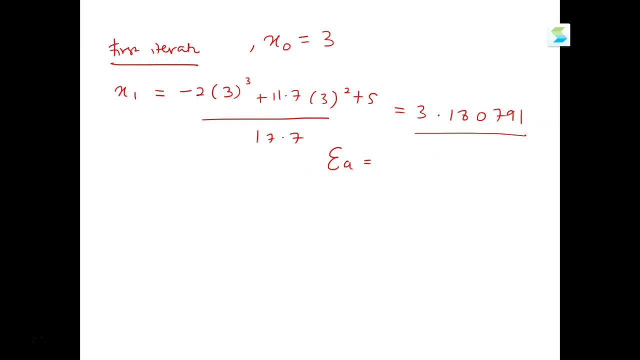 Because you have the value of your current answer And your previous approximation. So your EA is 3.180791 minus 3. Divided by 3.180791.. Times 100% And you should be getting 5.68%. 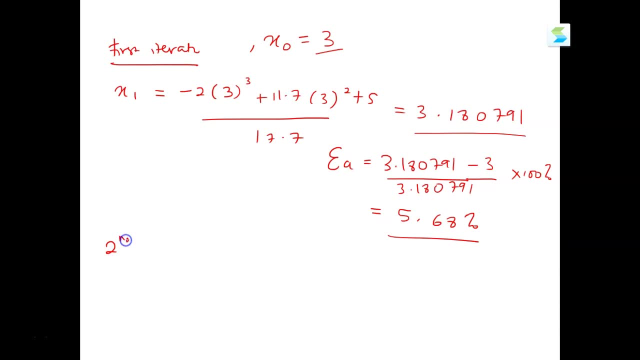 Next is your second iteration, So I will call it as x2.. So negative 2.. Okay, now For the x part. here We cannot use this value anymore. We have to use the newly calculated value. So you can use the newly calculated value.